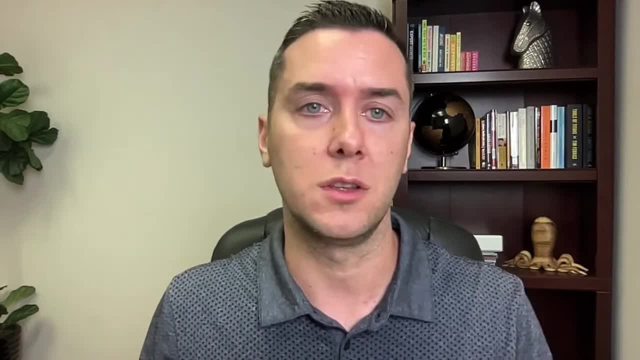 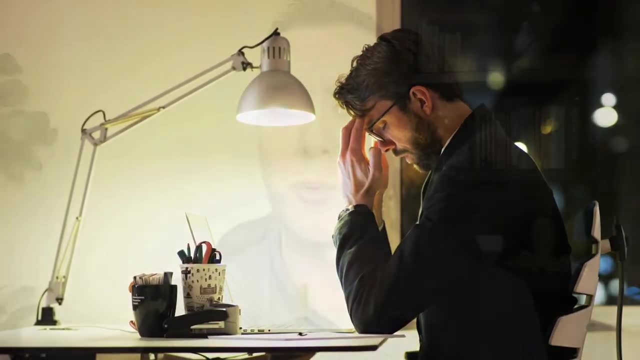 only way to get an accurate answer. So these questions might include about your stress levels, about your sleep habits, your education level. if you're optimistic or pessimistic about the future, all right. And then there's questions about your lifestyle, such as: how much coffee do you drink? 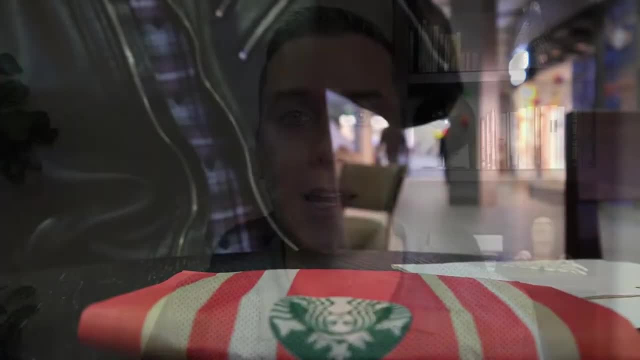 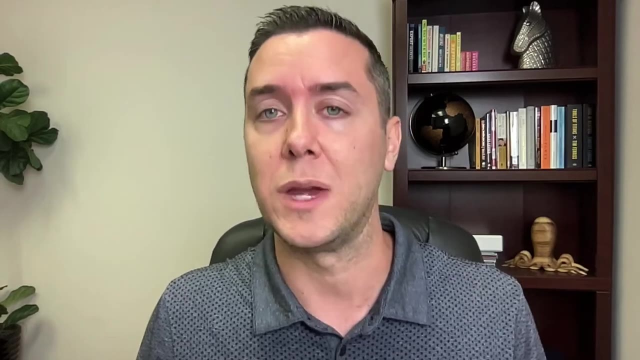 do you sleep? Do you smoke or are you exposed to secondhand smoke? Do you drink alcohol? Do you put on sunscreen? And then there's usually questions about your nutrition, your weight, how much red meat you eat, how much processed foods you eat, how much dairy you eat right, Et cetera. all these 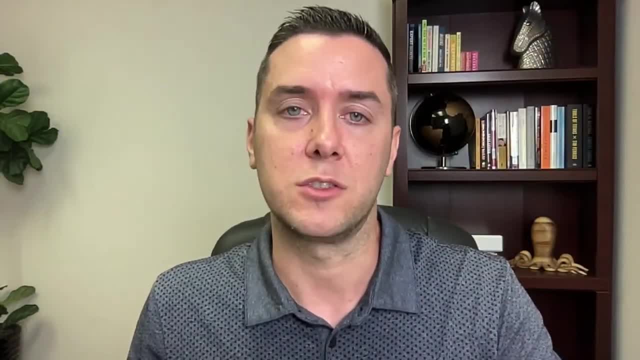 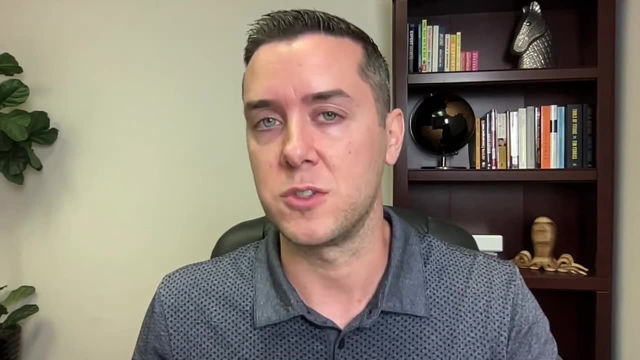 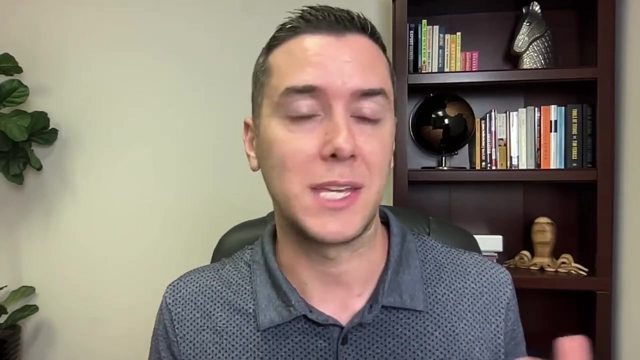 different questions. And then there's, finally, the medical history, right, Your medical history, your family's medical history, which can determine whether or not you are at risk for certain illnesses, right? So, if you're your, your family members, a sibling, a parent, had a certain illness, maybe cancer or stroke or heart disease, If they had some. 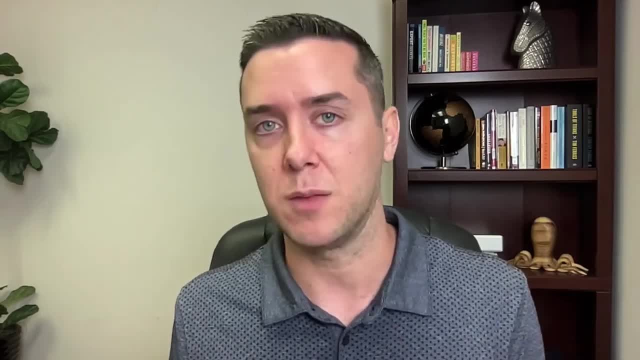 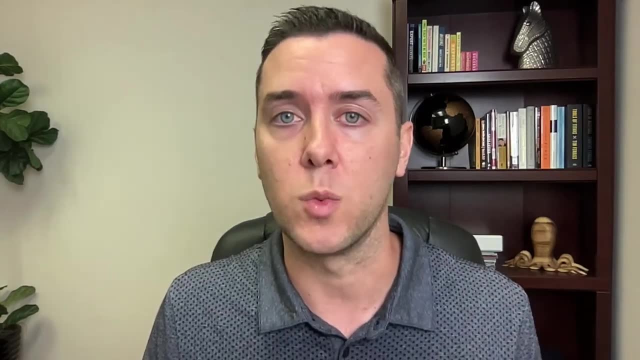 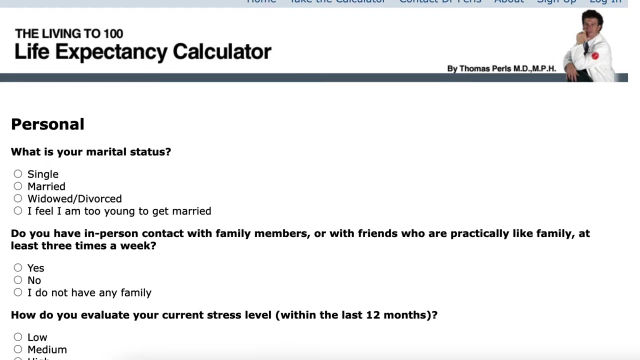 kind of illness, it's more than likely that it can run in the family, right. So my favorite online calculator to to actually determine your life expectancy is one called wwwlivingto100.com, And I will leave a link to this in the description below, And it was created by Dr Thomas Pearls. 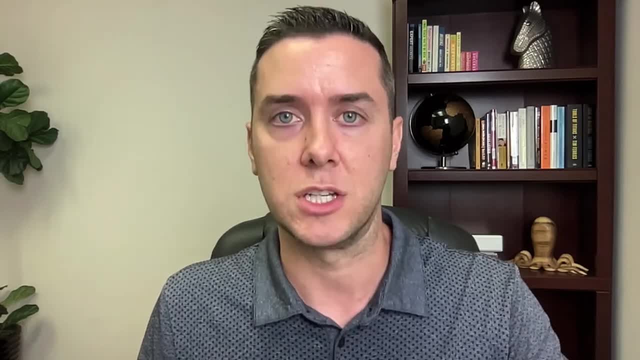 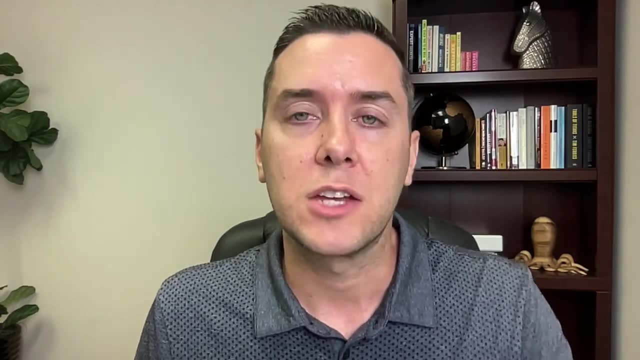 and I highly recommend it. It's a very thorough calculation based on these answers that you give And most people don't realize that you can actually add, you can actually do things in your life. make some simple changes that can. that can make a dramatic. 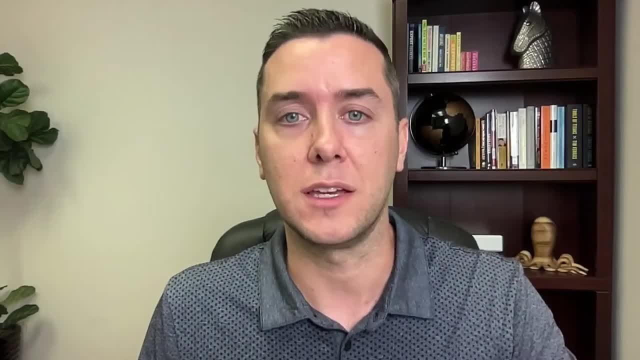 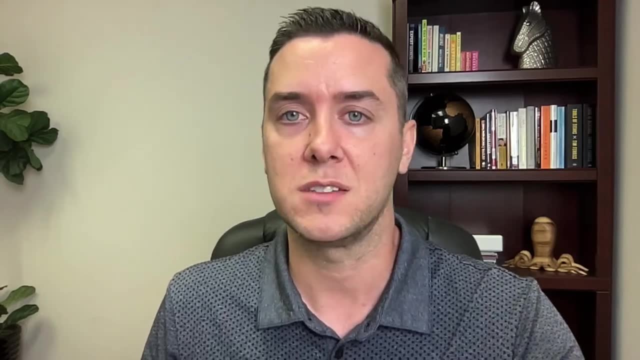 impact on your life, on the length of your life, And we're going to go over right now a study that was published in published library of science, medicine, And it shows us how we can actually add 10 years of like life expectancy. So in this new study, 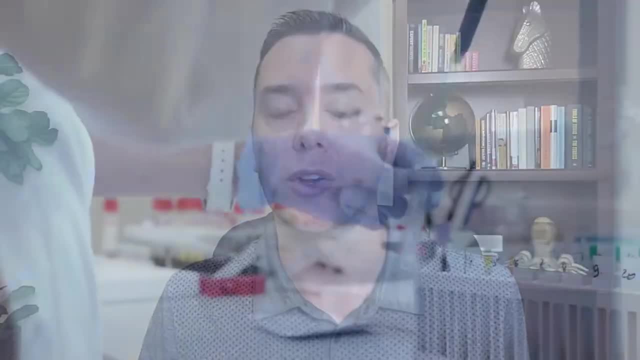 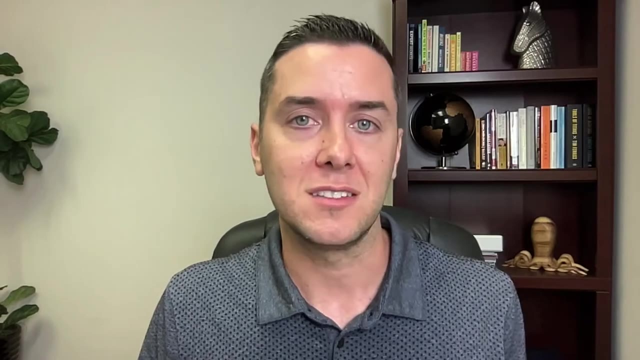 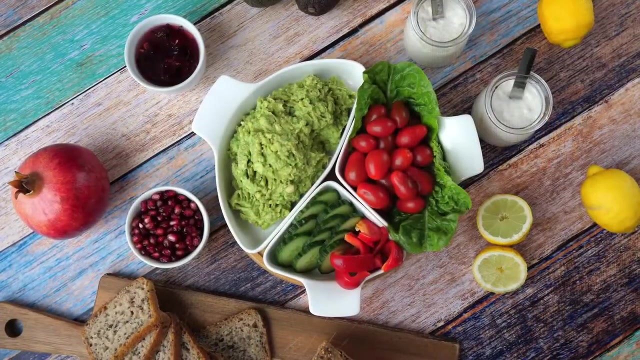 doctors use existing meta analysis and data from the global burden of diseases study to build a model, right? So this model actually enables the instant estimation of the effect on life expectancy for a range of different dietary changes, right? So what food we are consuming? 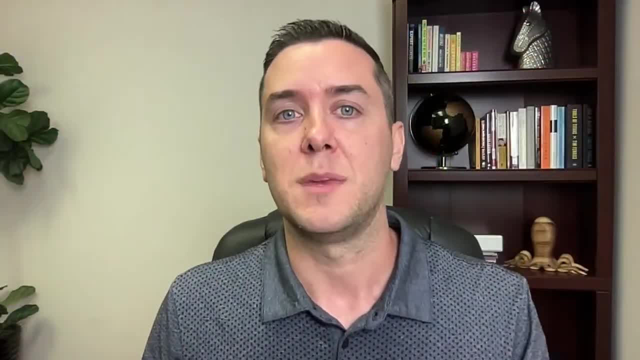 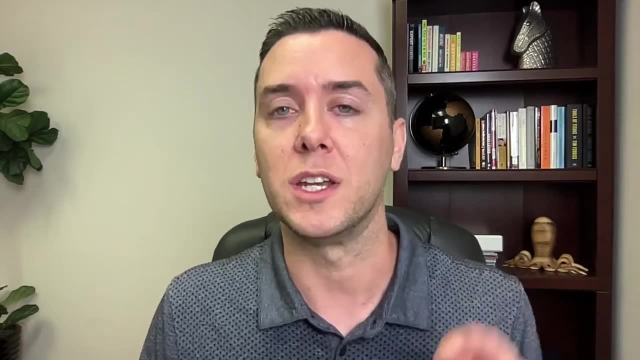 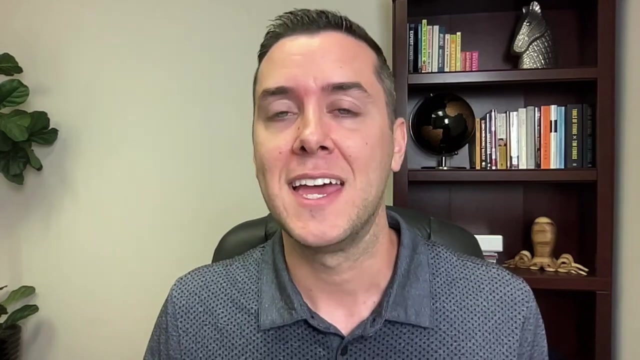 So for young adults in the US, the model estimates that a change from a typical Western diet to the optimal diet that they determined, beginning at the age of 20 would, would increase our life expectancy by more than a decade for women, right The average of 10.7 years and an average of 13 years for men. 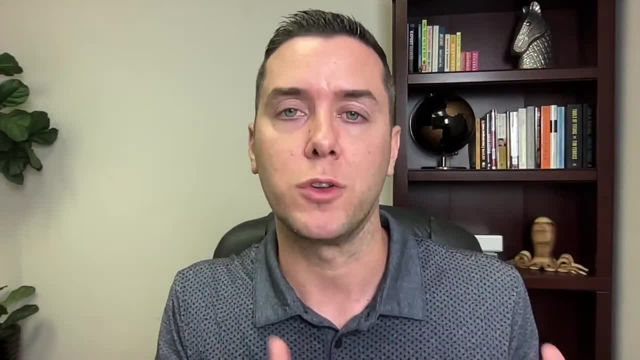 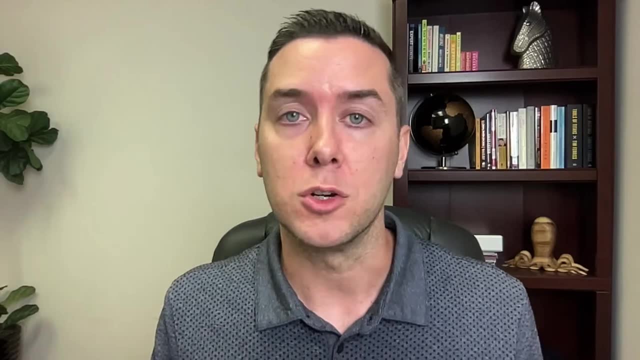 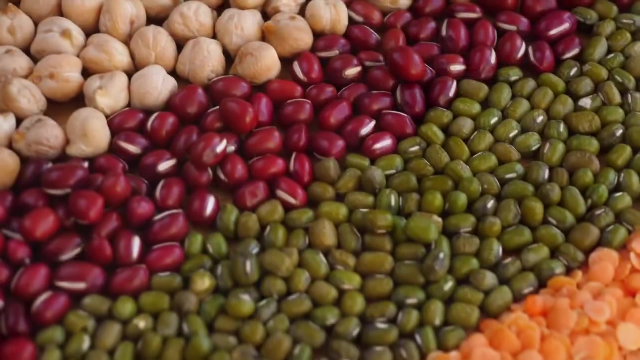 Mind blown right. Imagine making some changes early on in your life. that can add 10.7 years If you're a woman, or 13 years if you're a man, right, So the largest gains that they found in life expectancy would made are made by eating more legumes, more things like beans. 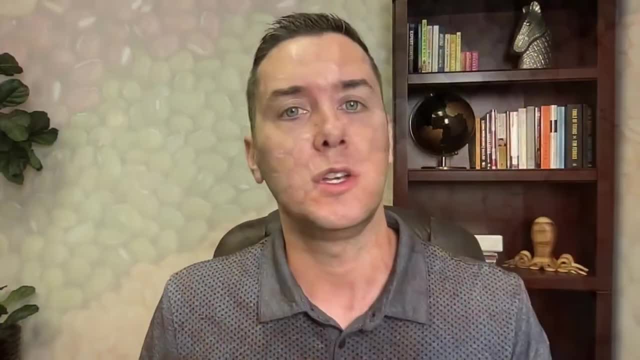 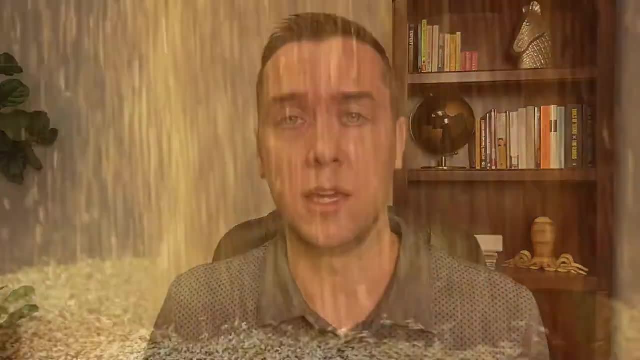 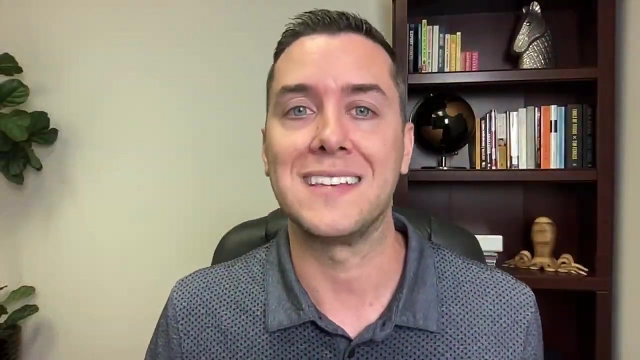 peas lentils right, Which they found would add 2.2 years on average for women and 2.5 years on average for men. And then next came whole grains: right, If you eat more whole grains, they expected you to live two years longer as a woman or 2.3 years longer as a man. right, More nuts can include. 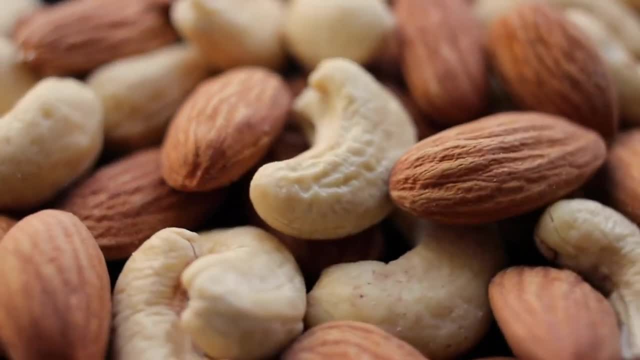 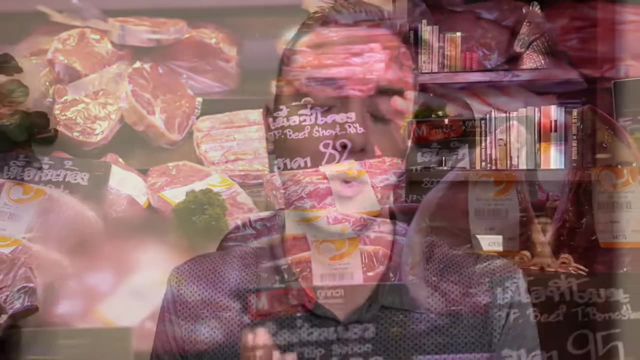 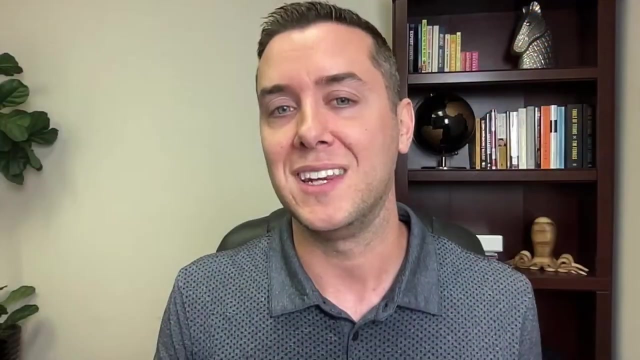 or including more nuts, would add 1.7 years for women, two years for men. Less red meat is 1.6 years for women, 1.9 years for men. Less processed meat would be 1.6 more years for women and 1.9. 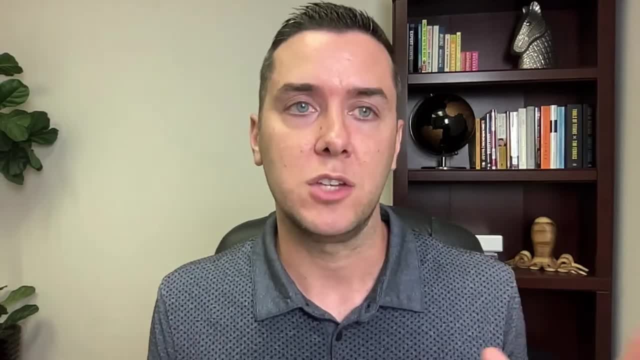 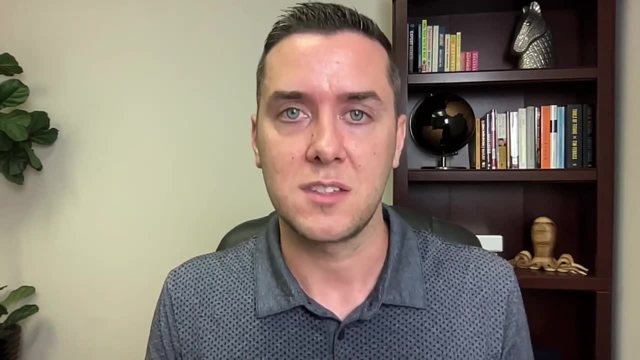 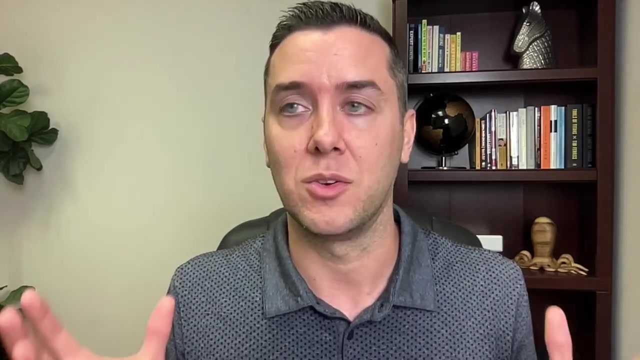 years for men. So this doesn't mean that you can change your diet overnight if you're 70 years old and you're going to add 10 more years to your life. This is this model is simply telling you that if you change your diet early in life, like in your twenties, and and you sustain this diet, 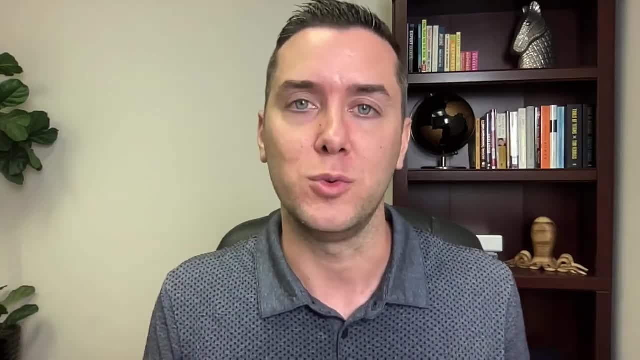 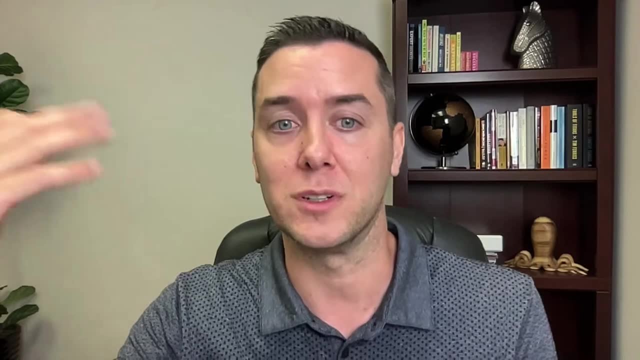 of adding more whole foods, more real foods, to your diet. you're going to be able to change your diet- less processed, less red meat- then you can have these advantages right. But they did find that if you were, let's say, 60 years old, you can still increase your life expectancy by eight years. 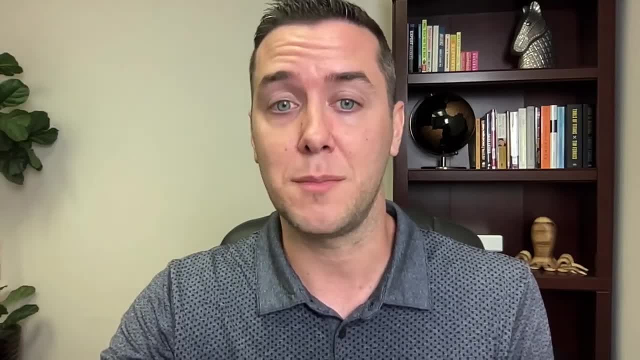 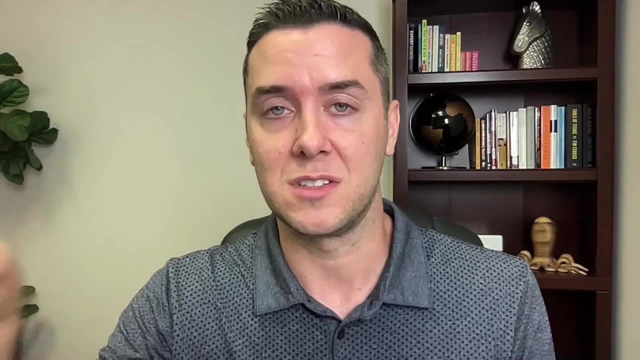 eight years as a woman and 8.8 years as a man. right, And let's say you're 80 years old. they found that you can gain 3.4 years for men and women with such dietary changes, right? So this model is how we should think about our life expectancy. 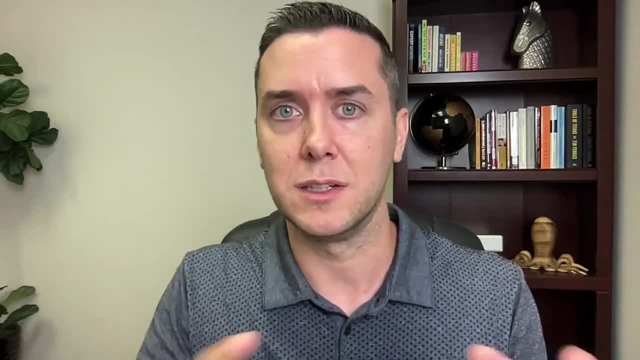 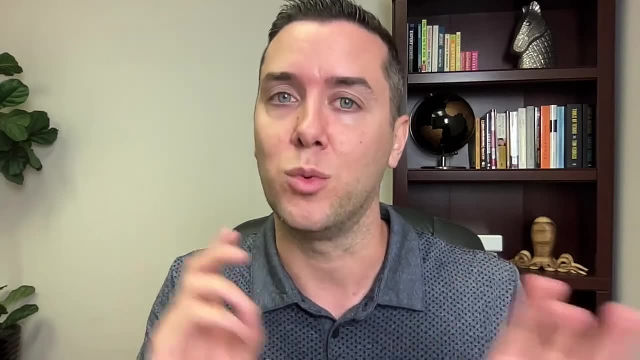 and increasing it and increasing it. I'm going to leave a link to the study and to the actual model below where you can fine tune what you, what you know, your diet and what would be the optimal diet for you. All right, So I'll leave a link to that in the description below. I'm also 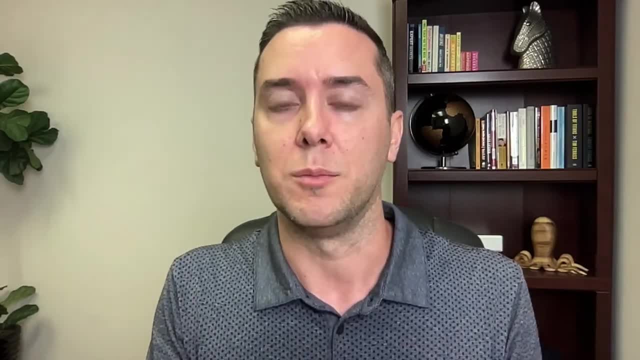 going to leave a link to the calculator living to 100, uh, below for you to check out. And, um, I hope this was insightful for you, I hope it was helpful for you, Uh, and if you did like it,